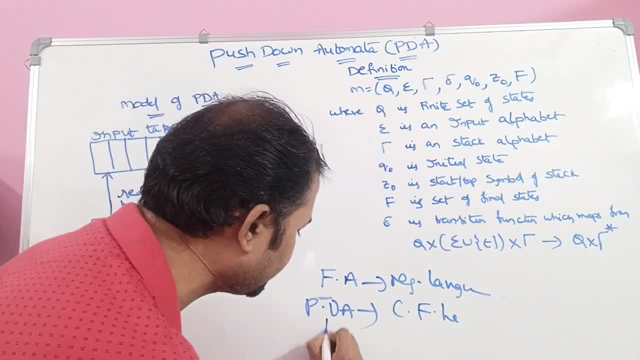 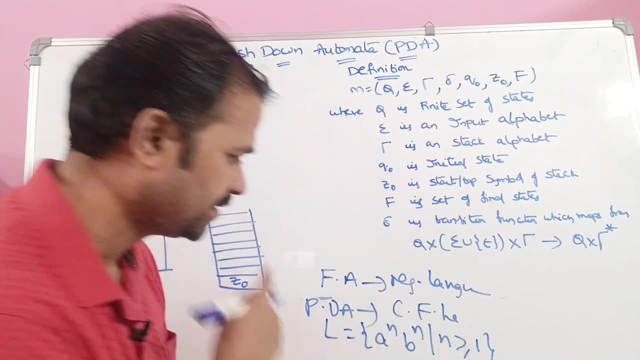 Let us take an example. Let we have a language called L is equal to a power n, b power n, such that n is greater than or equal to 1.. So here, number of a's, n. number of a's are followed. 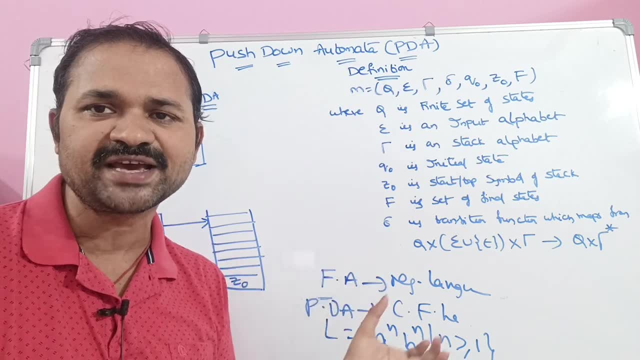 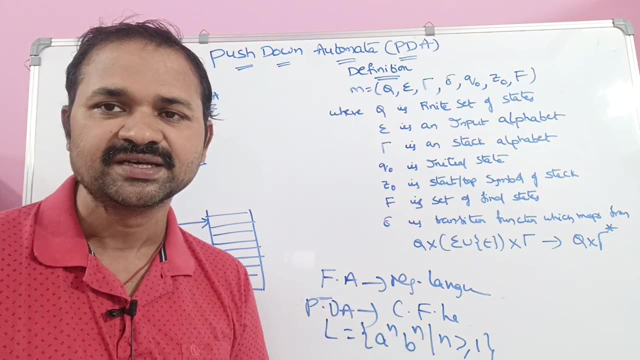 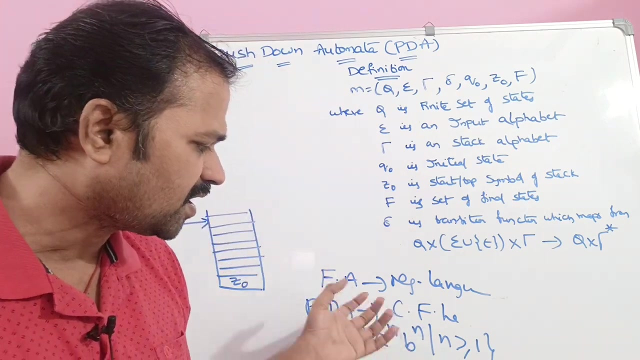 by n, number of b's. So here the number of a's and number of b's must be equal, And number of b's, number of a's, are followed by number of b's. So here, in order to, by using finite automata it cannot recognize- 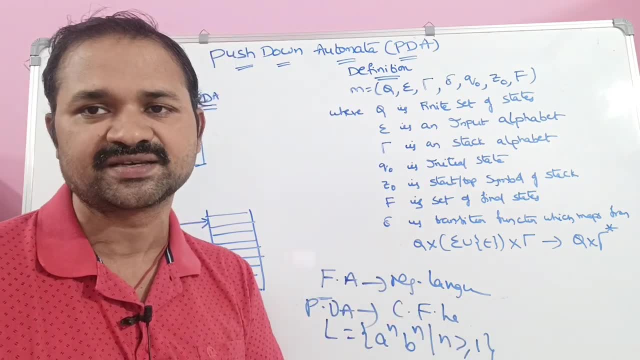 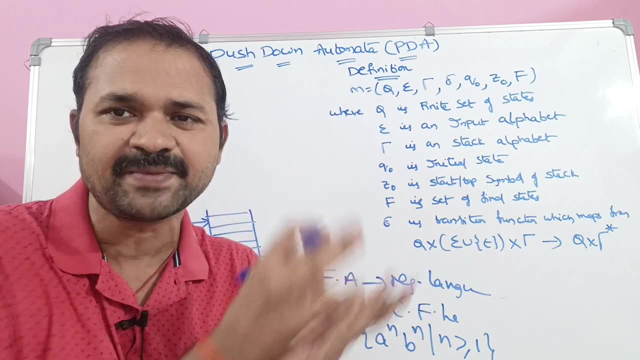 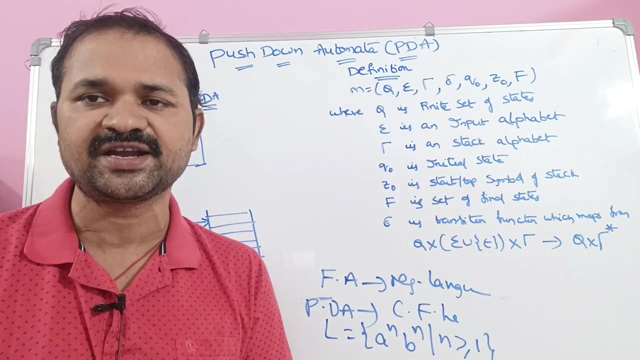 this language. It cannot be a regular language. Why? Because here number of a's and number of b's must be equal, So we should have some comparison mechanism. But that comparison mechanism is not there in finite automata. So this is the problem with finite automata. 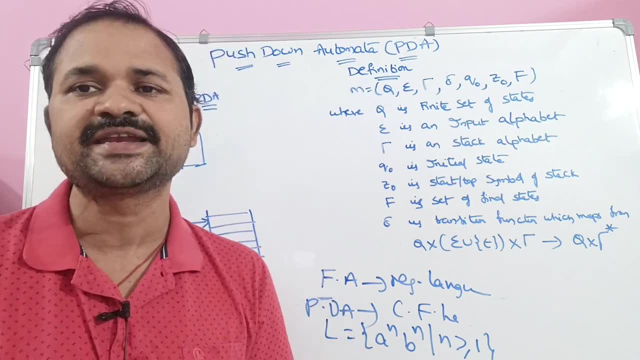 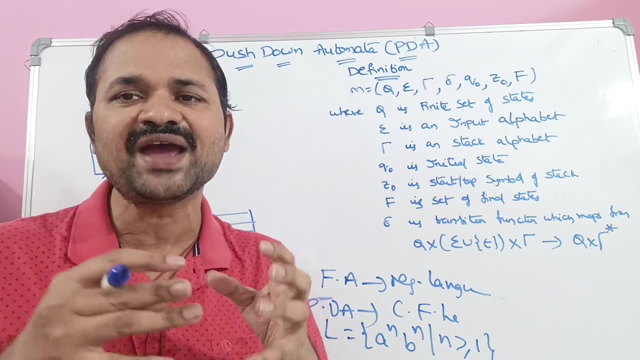 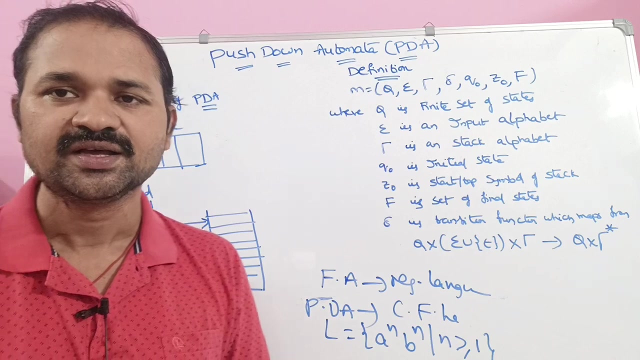 Finite automata has finite amount of memory. It can store only limited piece of information. If we want to store some complex languages, if we want to handle some complex languages, then it is not possible with finite automata. The best example is this example: Here we need: 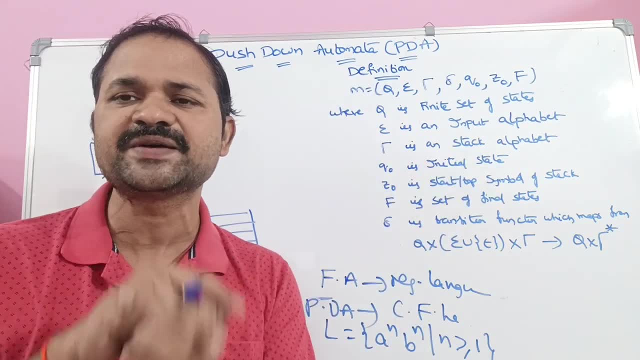 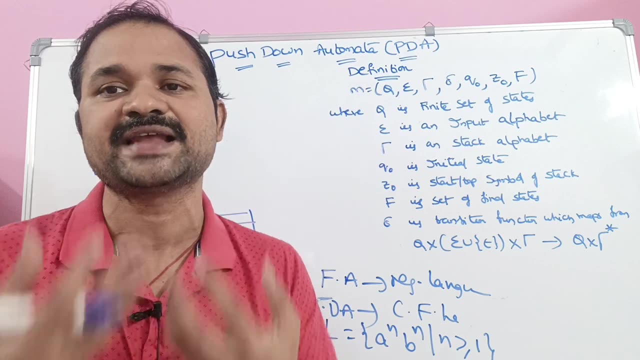 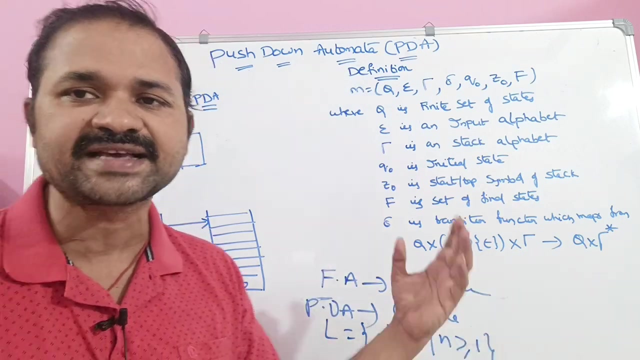 some comparison mechanism. Number of yes and number of this must be equal. but that comparison mechanism is not there in finite automata. So if we want to handle complex languages, then we have to go for context-free languages. and context-free languages are accepted, or? 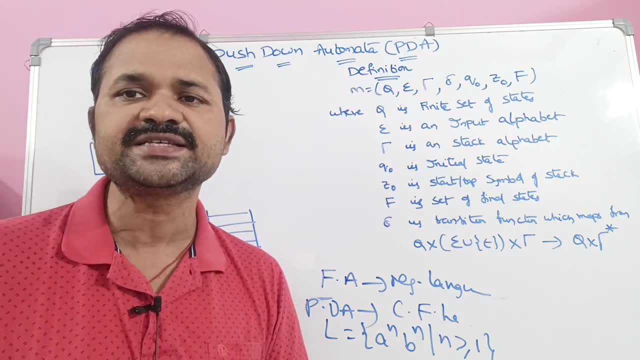 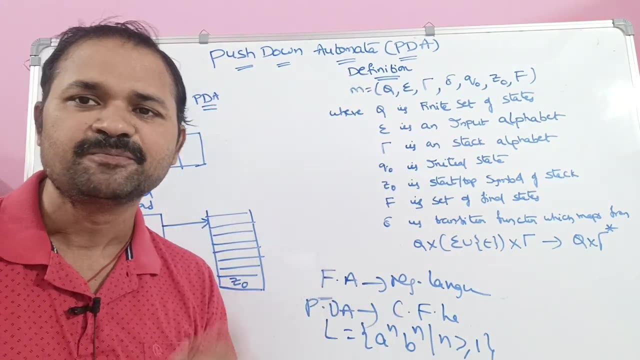 recognized by pushdown automata. Now let us see the model for the pushdown automata. Pushdown automata diagram. this is the model is nothing but pushdown automata diagram. Pushdown automata mainly contains three components. The first one is the pushdown automata diagram. The second one is the pushdown automata diagram. 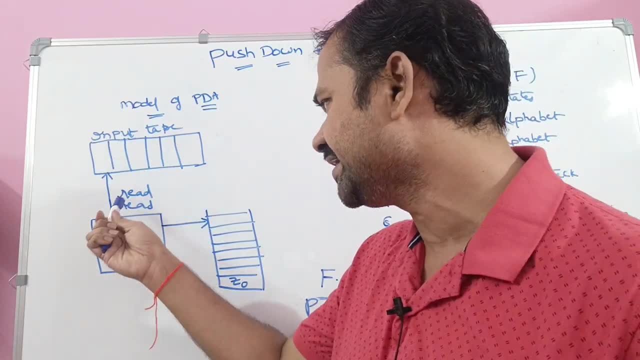 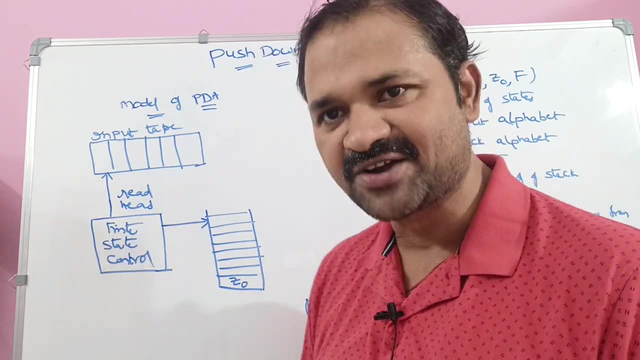 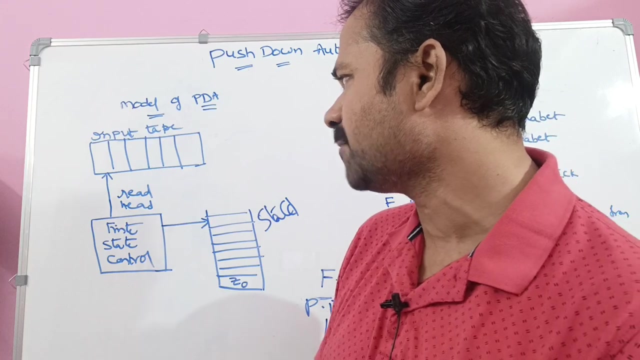 The first component is input tape. The second component is finite state control. So this is nothing but finite control machine, That is nothing but finite automata. And third component is stack. Third component is stack. So what is the first component? Input tape. 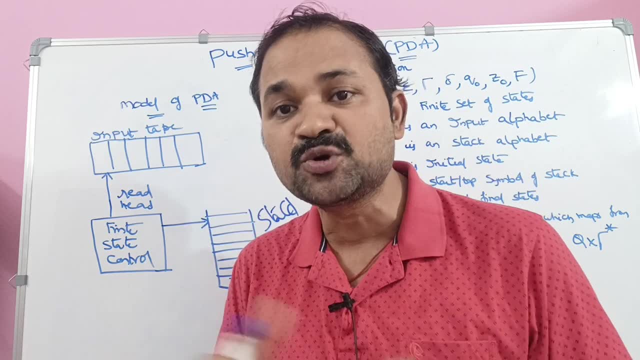 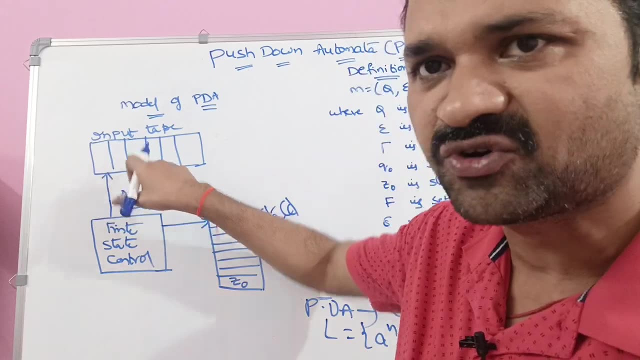 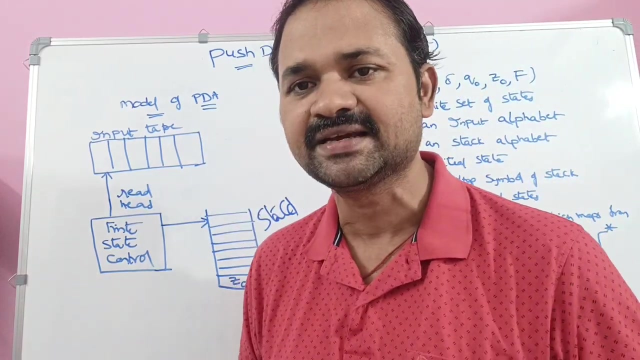 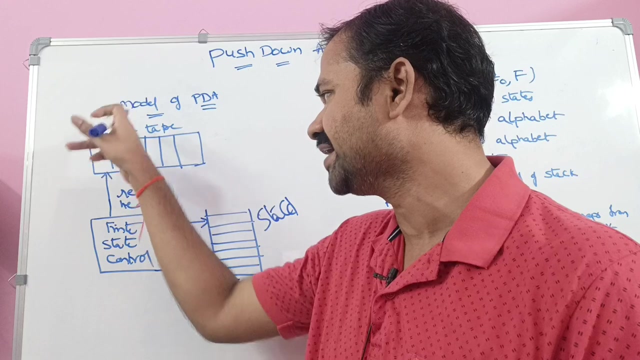 Input tape is mainly used for storing the input string. Here the input tape is divided into number of cells. This is the first cell, second cell, third cell, fourth cell. like that, Input tape is divided into number of cells, where each cell can store one symbol at a time. 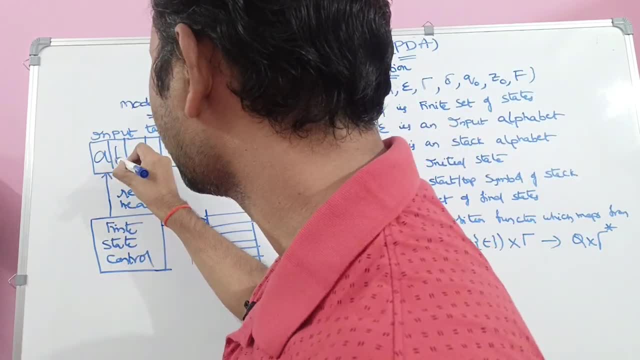 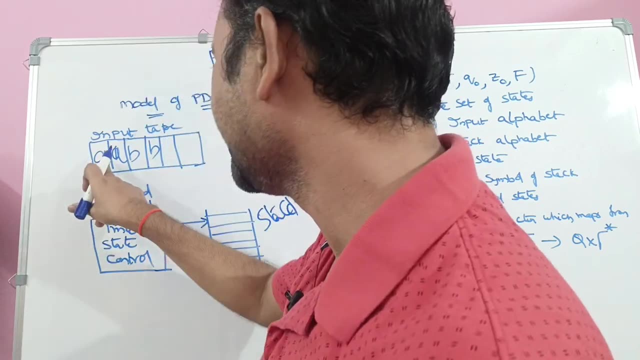 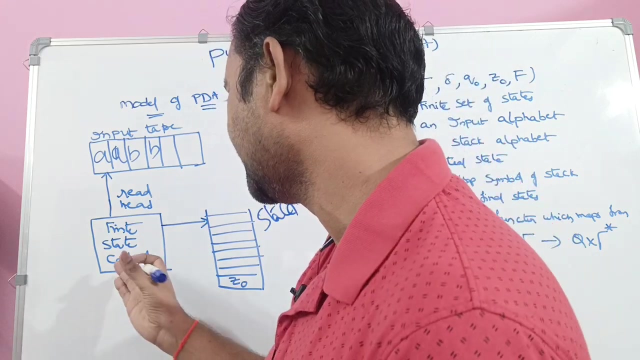 Let me have a string like this: a b a, a b b. So a a b b. Let us assume that this is the string, So each cell can store only one symbol at a time. So we have a a b b. Next the second. 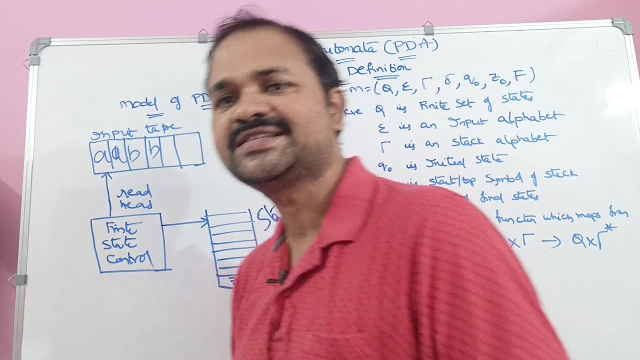 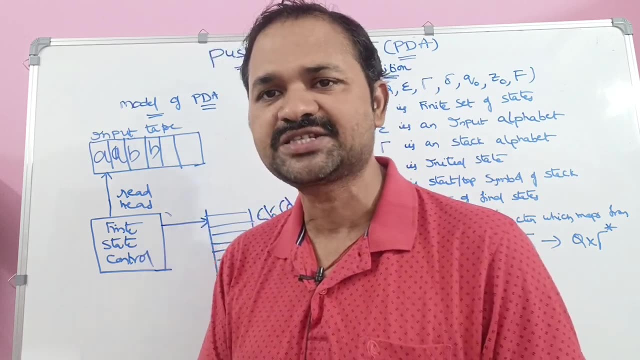 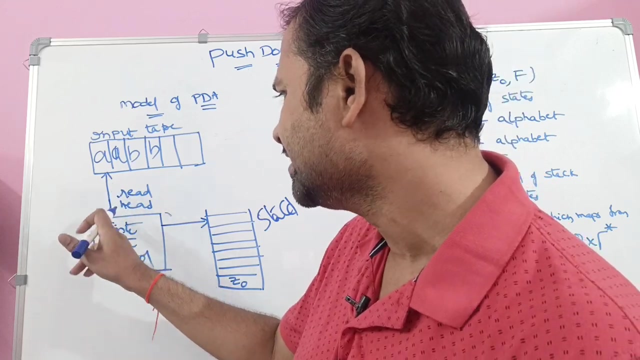 component is finite state control. So this is nothing but finite automata, finite control machine. So it contains a finite set of states, So all the states are available here, And it maintains two heads. So read head. read head points to the first symbol of the input tape. 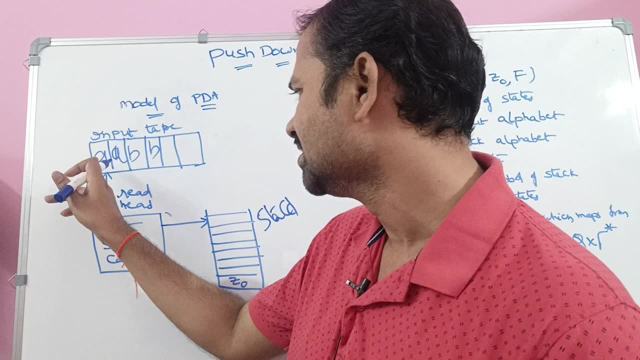 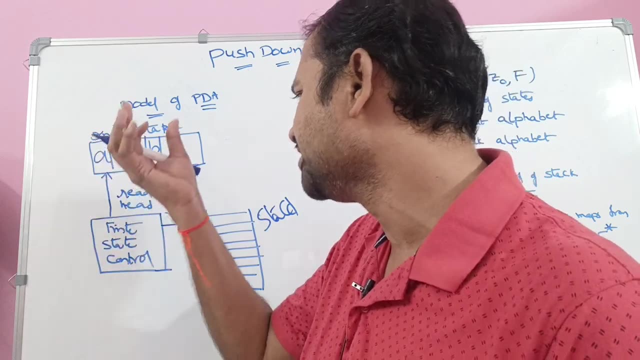 It points to the first symbol of the input tape. So it points to the first symbol of the input tape. Read head always points to the first symbol of the input tape. So first the symbol will be read head After reading that symbol and it moves the read head in forward direction. So that means 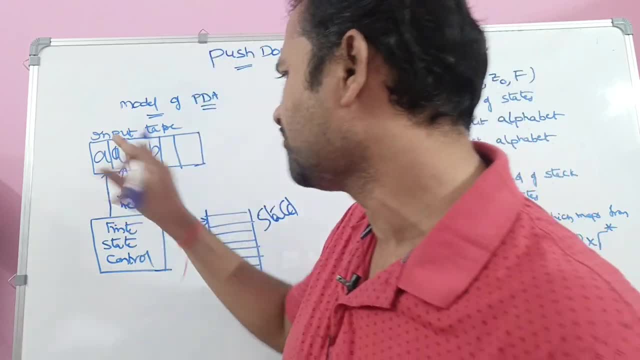 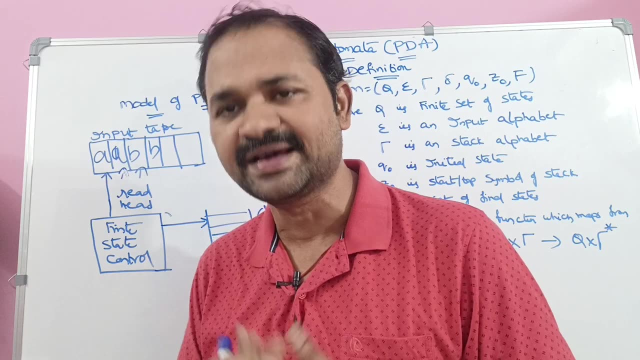 next read head will points to this cell. So after reading this cell, then the read head will points to this cell. So likewise, symbol by symbol, the data will be read head. So this is about finite control machine Here. the difference between finite control machine and finite control machine is that 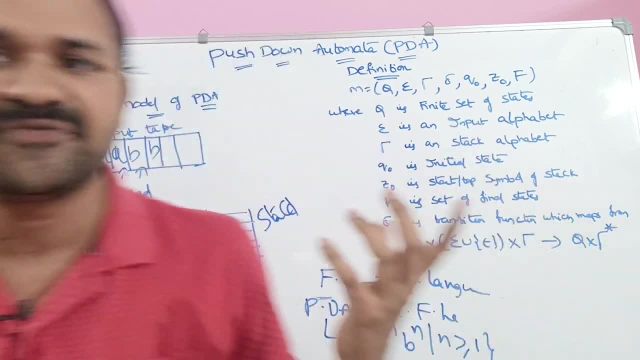 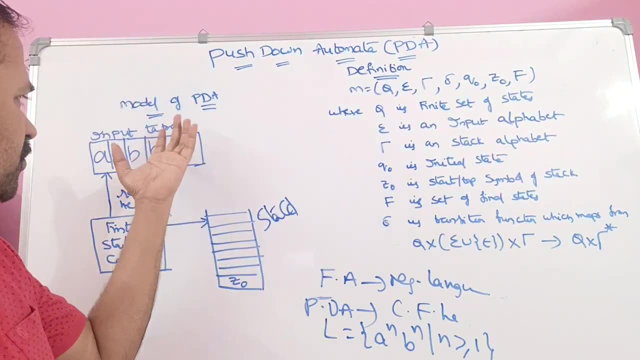 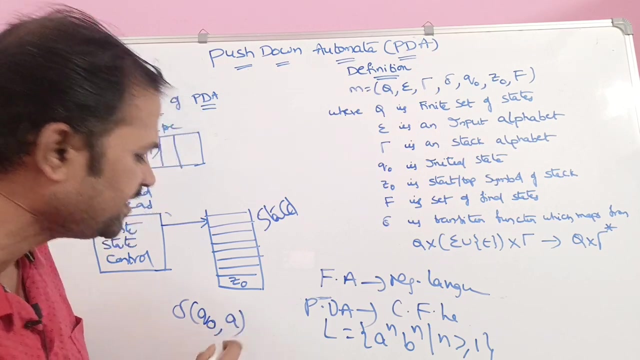 here the difference is: in finite automata we have only input tape as well as finite state control, So depends upon the input symbol. by applying input symbol on a state, let the state is q. naught, let the input symbol is here. By applying input symbol on a state, we will go to. 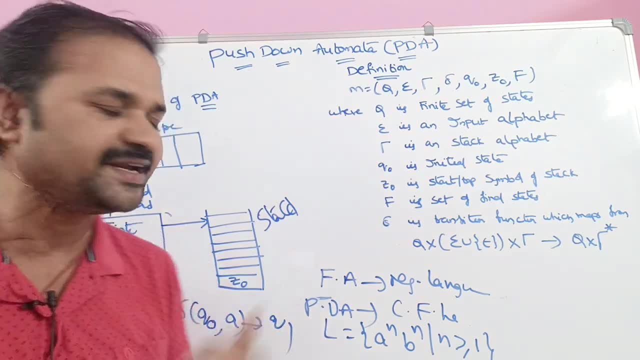 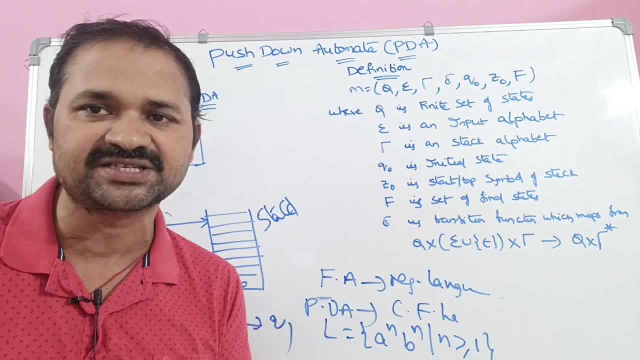 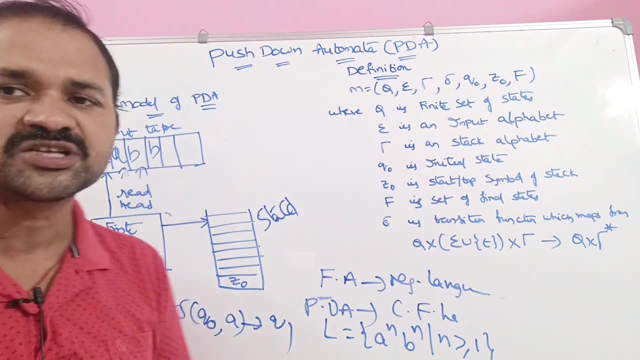 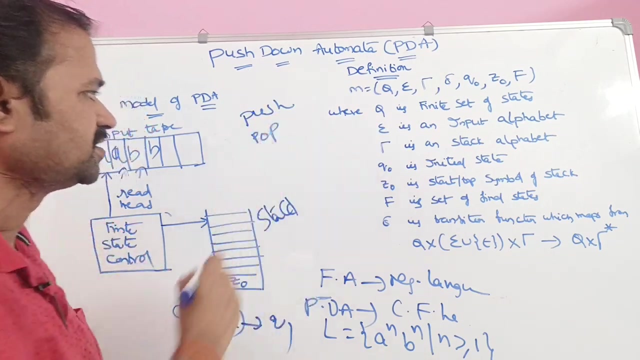 know what is a stack. It is a data structure. It is used for storing the elements. Here, the elements are nothing but symbols. It is used for storing these input symbols, Symbols. On stack. we can perform two operations. The first operation is push operation. The second operation is pop operation. 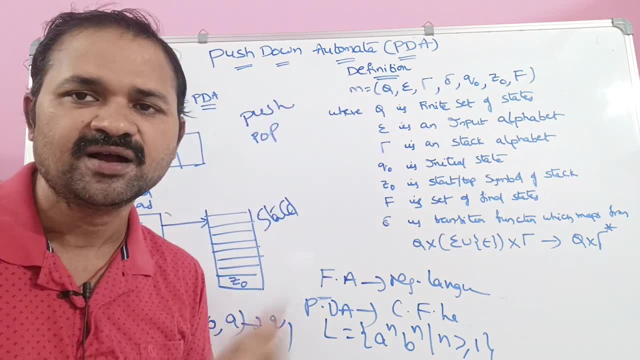 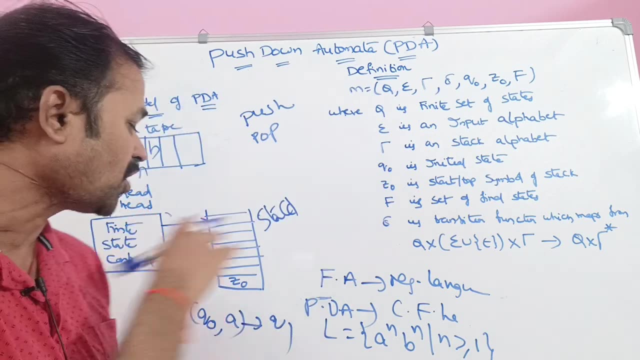 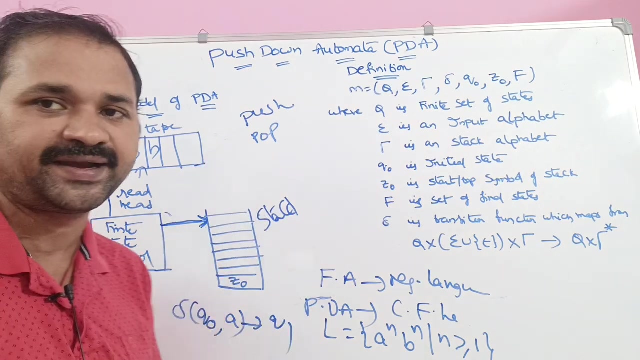 So push operation pushes the symbols onto the stack. Pop operation pops the symbols from the stack. Always, push operation and pop operation will be performed from top of the stack, Top of the stack. So that's why the second head will always points to the top head. Top head, Let the topmost 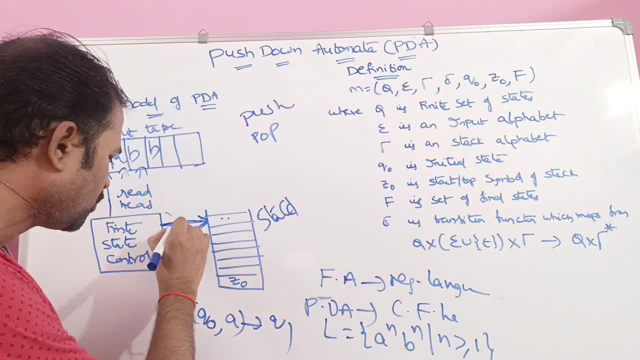 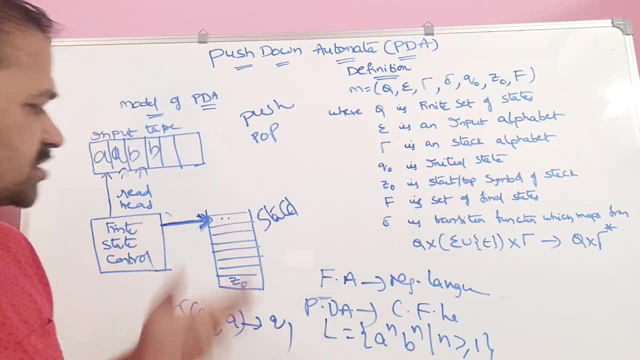 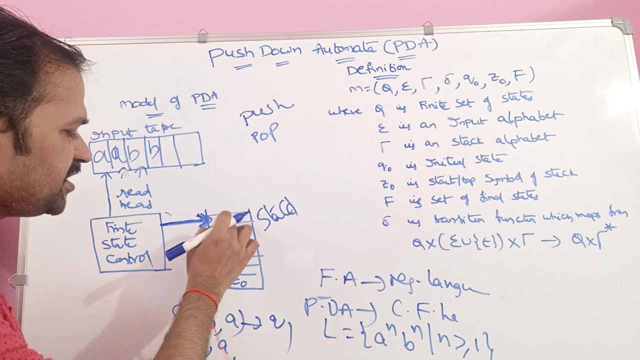 item is available here. So the finite control, the finite state control head, the second head always points to this stack's topmost item. Okay, So here, in addition to the, in addition to the input symbol we need to apply, we need to apply another symbol on the stack. 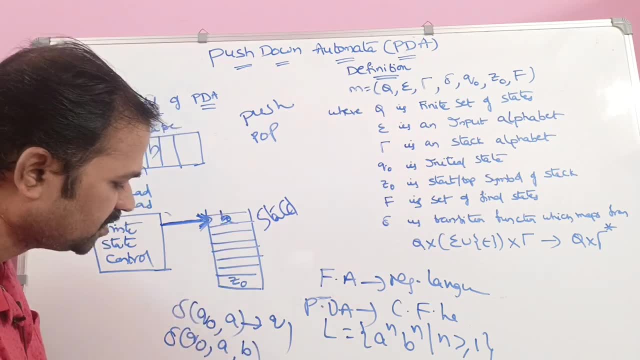 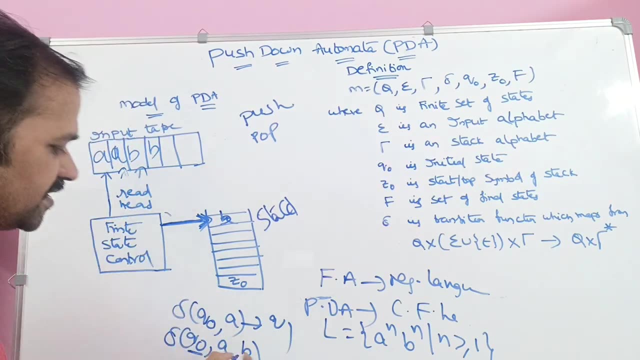 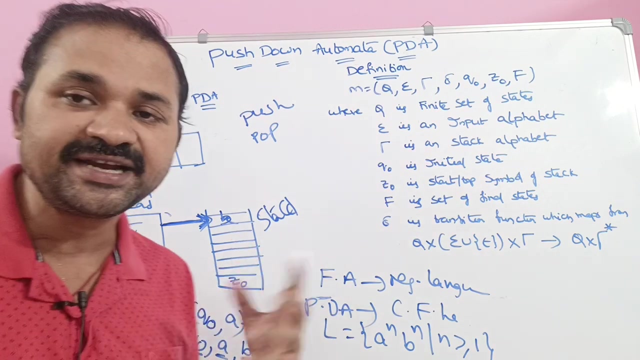 That is stack's topmost symbol, Let the symbol is B. So here, this is the current state. This A is nothing but this input state, input symbols, whereas this B- this B is nothing but stack's topmost symbol. So here on the state, in addition to the input symbol, we need to apply this one: 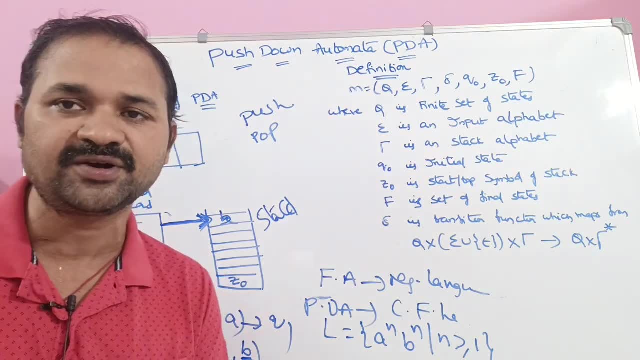 also. This is nothing but stack's topmost symbol. Okay, Here we have Z naught. Z naught is nothing but stack's topmost symbol. So here we have Z naught. Z naught is nothing but stack's topmost. 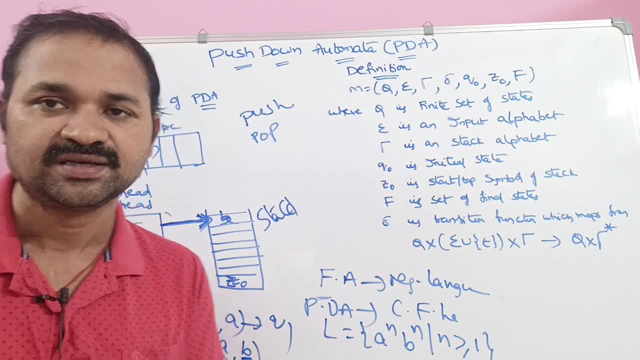 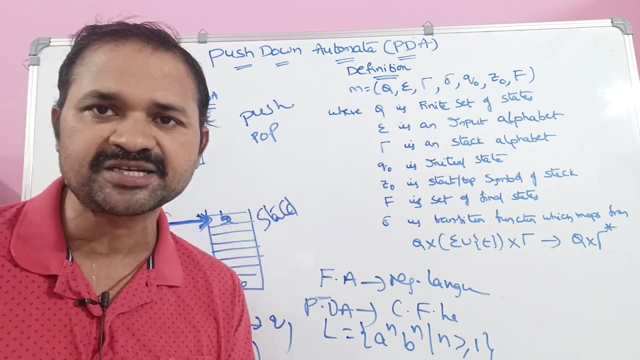 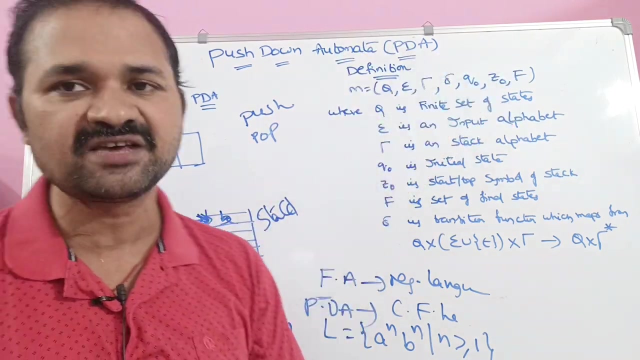 symbol, or this can also be called as start symbol. So Z naught means stack's topmost or start symbol. Here stack produces mainly two states, either accepted state or rejected state. Now let us see the definition of the PDA. PDA is defined by seven tuples. The first tuple is Q. 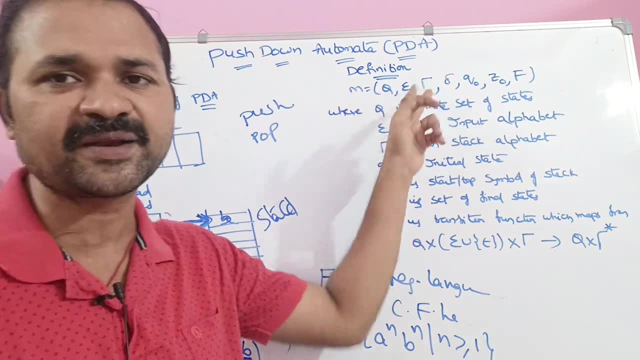 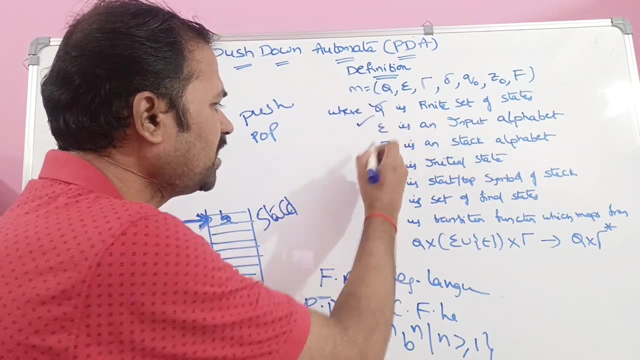 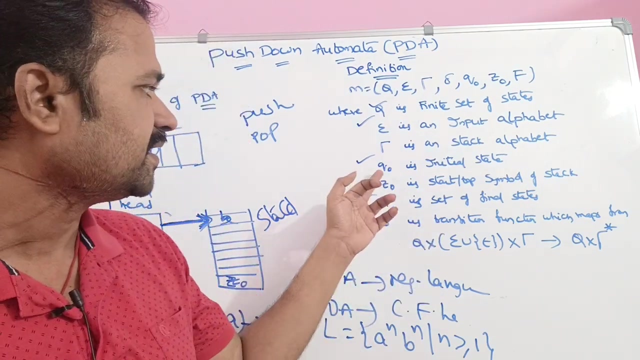 second tuple is sigma. third tuple is tau. This is pronounced as tau. Next one is delta: Q naught Z, naught F. So we know about Q, sigma, Q naught F and delta also. So sigma is nothing but an input alphabet. And what is the second? 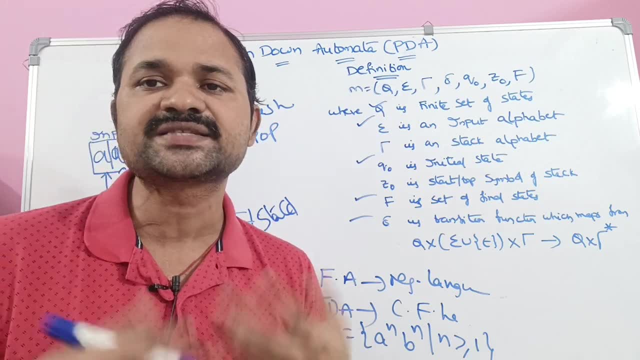 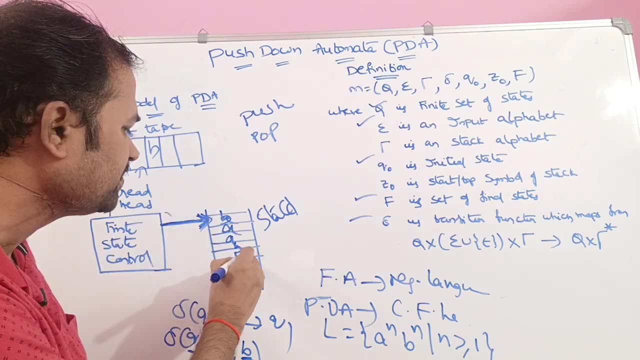 symbol Tau. Tau means stack alphabet, Tau means stack alphabet. Let us assume that here stack alphabet contains several symbols like A, B A B, B, A, B, A, B A B. So this is nothing but. 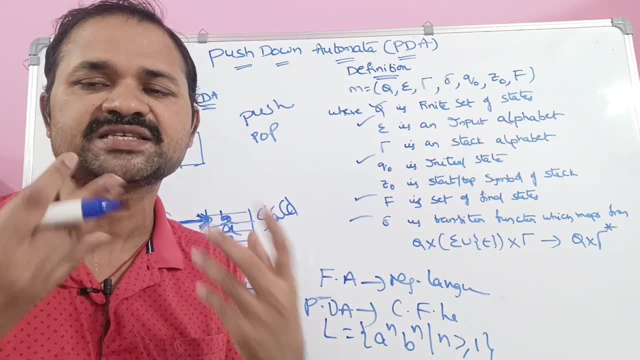 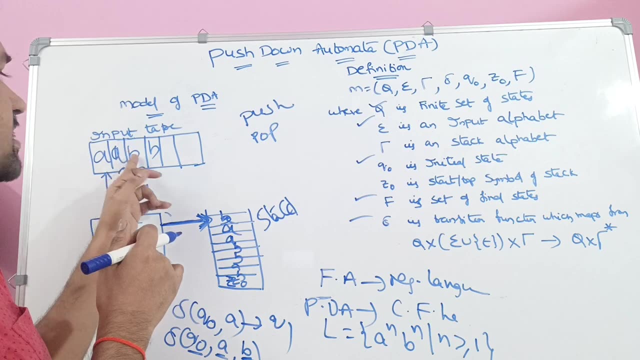 stack alphabet, stack alphabet symbols. So what are the symbols that are stored in the stack? So that is specified by tau symbol, And this is nothing but what Sigma. Sigma is nothing but what Input alphabet symbols. So next one is Q naught. 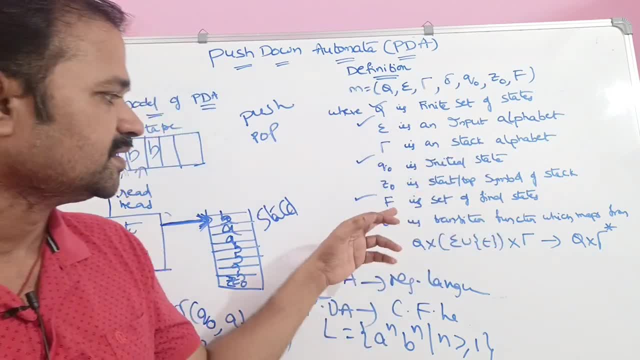 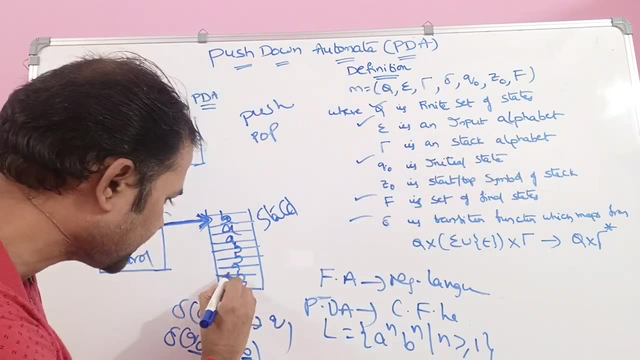 Q naught is nothing but initial state, just like the finite automata. Next we have Z naught. Z naught is nothing but starting or top symbol of the stack. So here we have Z naught. So 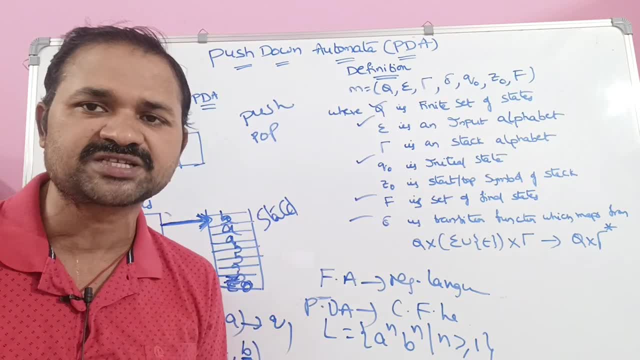 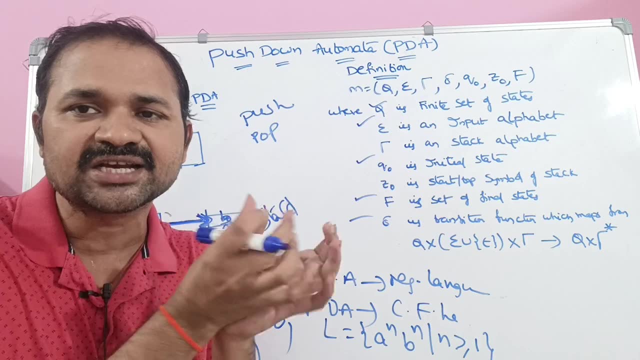 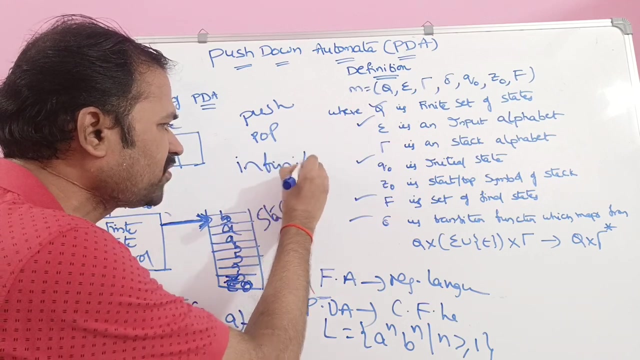 this Z naught is called as starting symbol or top symbol of the stack Here. one more advantage of the stack is: here the stack size is infinite, unbounded. We can store any number of symbols in the stack. So here the stack size is what: Infinite, So we can store any number of symbols. 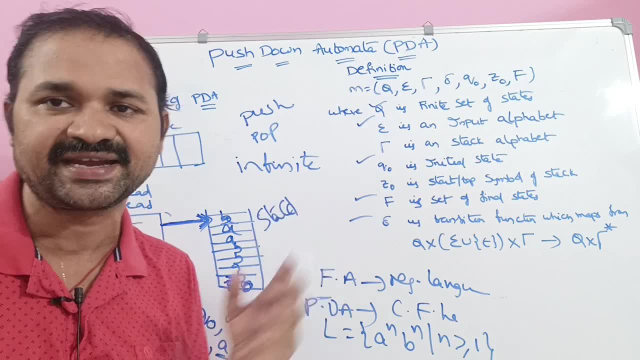 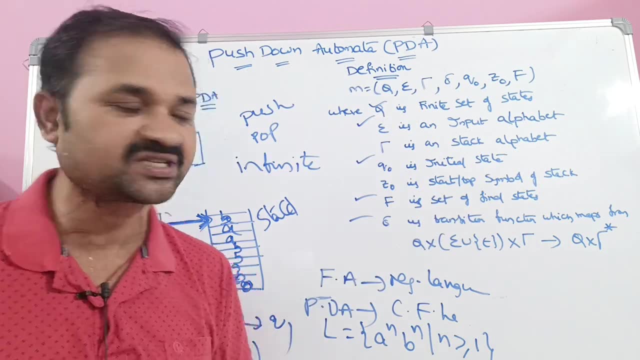 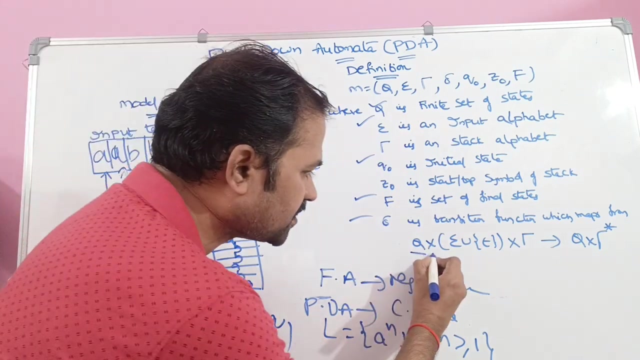 in the stack. So here the stack is not finite, It is infinite. The size of the stack is infinite. Next we have F. F means set of final states. Next one is what Delta? Delta is a transition function which maps from Q cross. And what is the second one Here? the second one is this input: 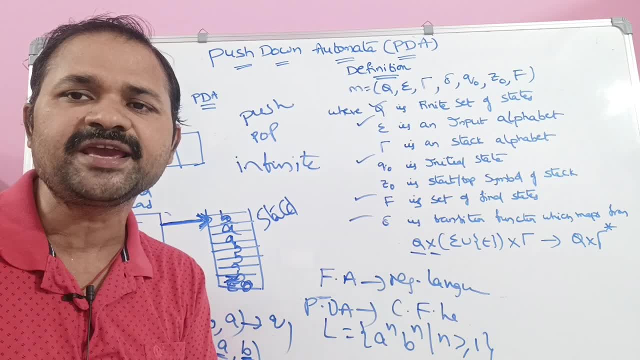 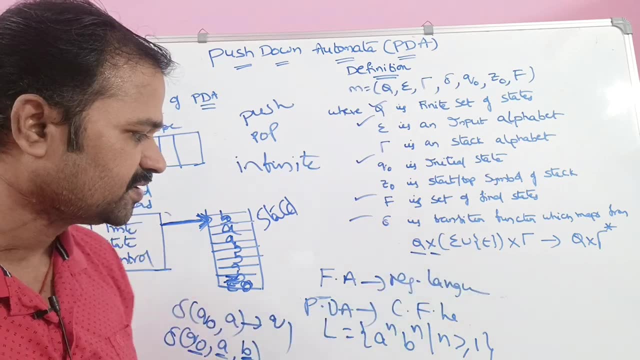 alphabet symbols: Sigma, Or without applying input symbol also, we can make the transition So: sigma union within the curly braces, epsilon. If we take the example here. let the Q naught is the state A, So here: 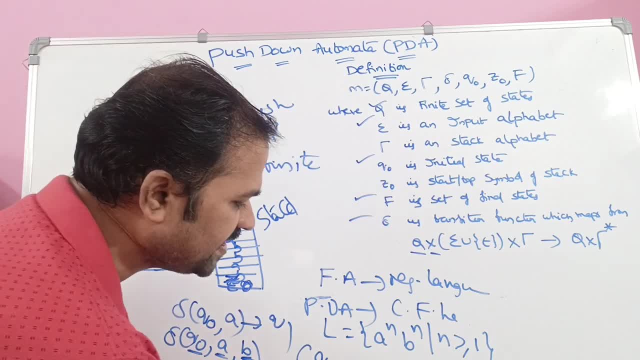 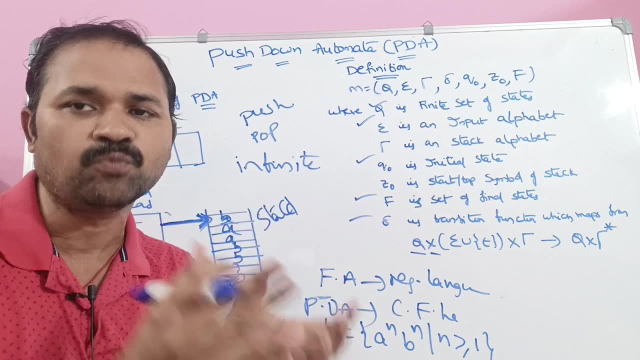 we have A. A is nothing but sigma. Or we can have epsilon also. Epsilon means without applying any symbol, without applying any input symbol also, we can make them move. So Q cross, sigma, union within the curly braces: epsilon. 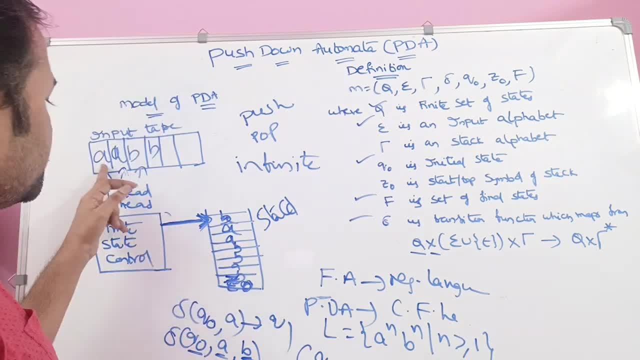 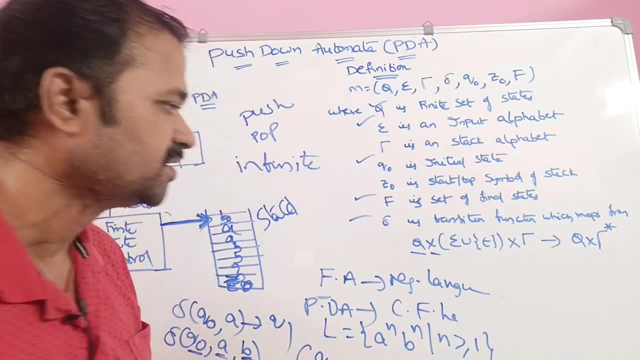 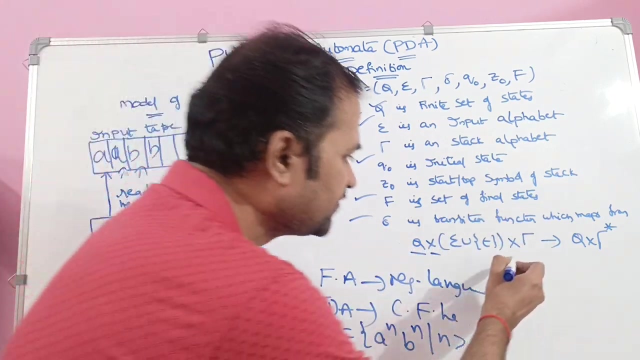 Cross. this is nothing but tau symbol. Here, in addition to input symbol, we need stack's topmost symbol also. Let, the stack's topmost symbol is B, So this B is nothing but tau symbol Implies. so delta is a transition function which maps from this current state to next state. So